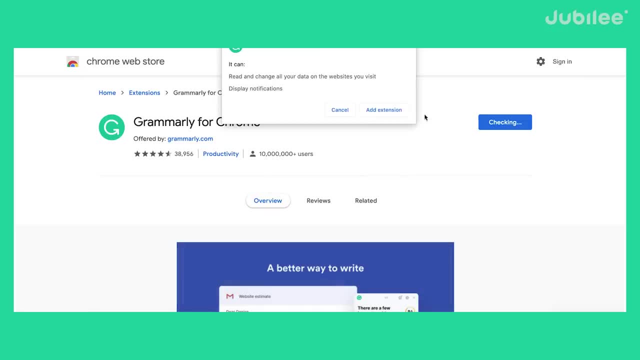 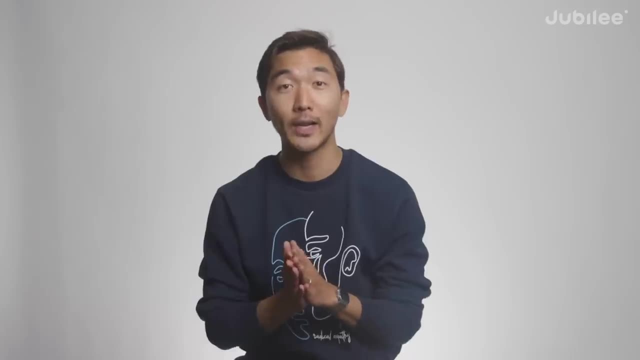 extension is super simple to download. Just go to grammarlycom and click install. now That's it. The free version of Grammarly has basic grammar and spelling suggestions, but upgrading to premium is totally worth it, And here's why Grammarly helps make vocabulary suggestions to make your 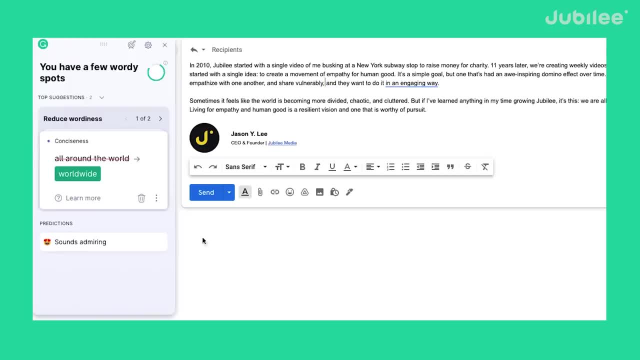 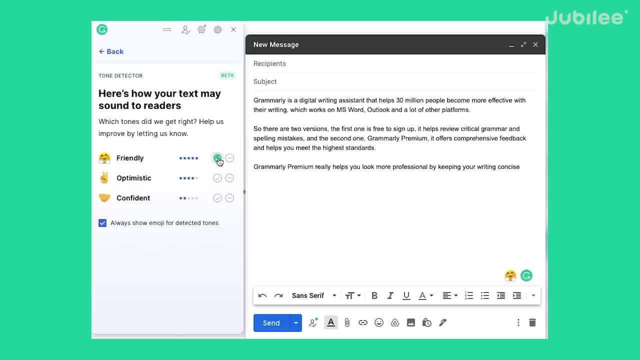 writing more exciting and effective. It also makes clarity suggestions so you can make your writing more concise. Finally, Grammarly helps you with the tone of your writing and provides a little feedback on whether or not your writing sounds professional. Go to grammarlycom slash. 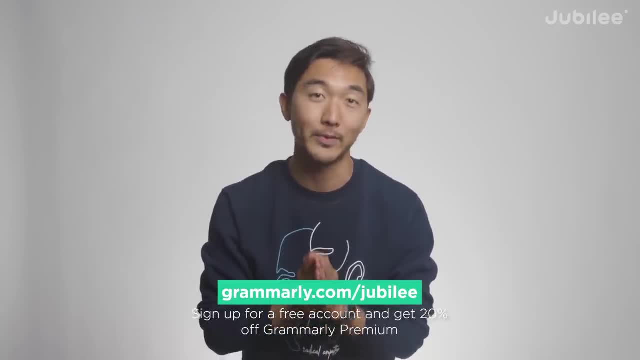 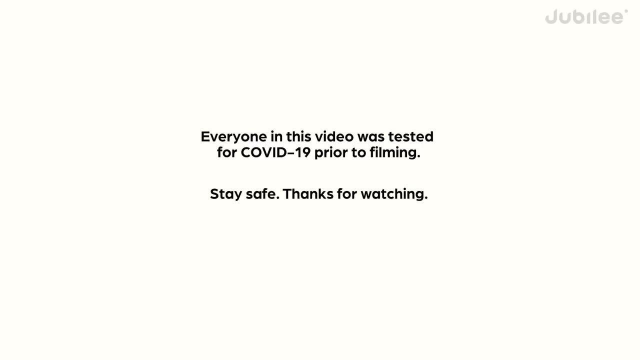 Jubilee to sign up for a free account and get 20% off Grammarly premium. today, Again, that's grammarlycom slash Jubilee. Now enjoy the episode. I wasn't planning to go to college. That wasn't like a. 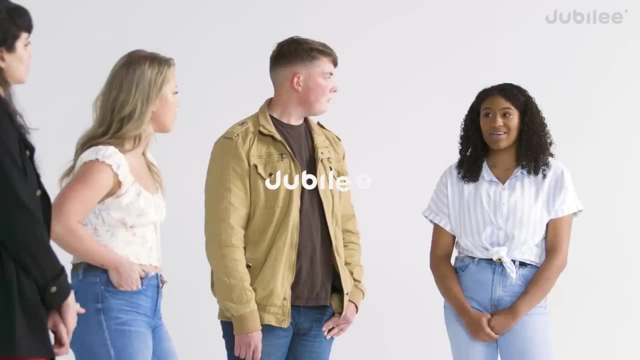 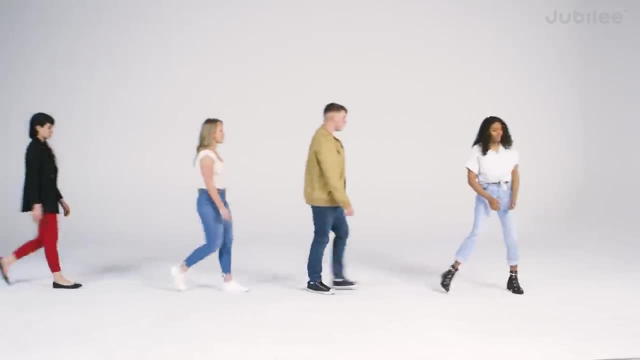 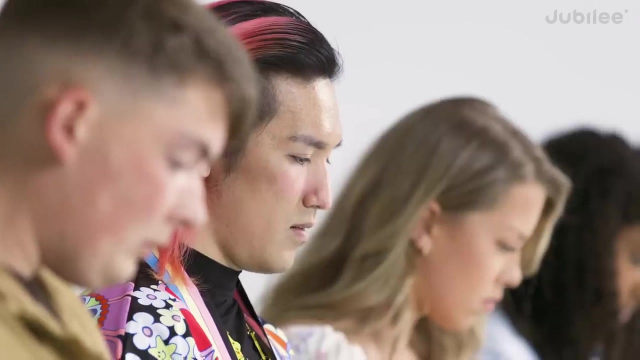 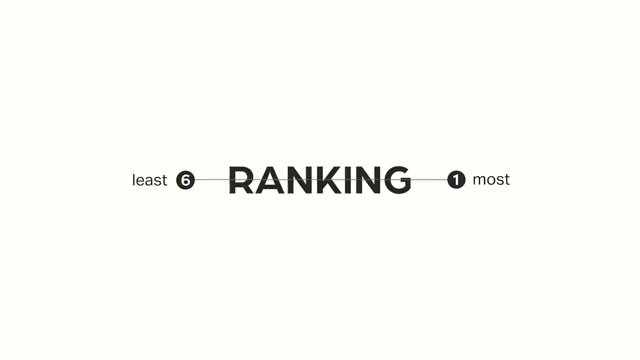 goal of mine. My parents were like, well, you should apply to at least one college. And I was like I'll never get in here. And then I went to Yale. Should we just like go down and do intros? Yeah? 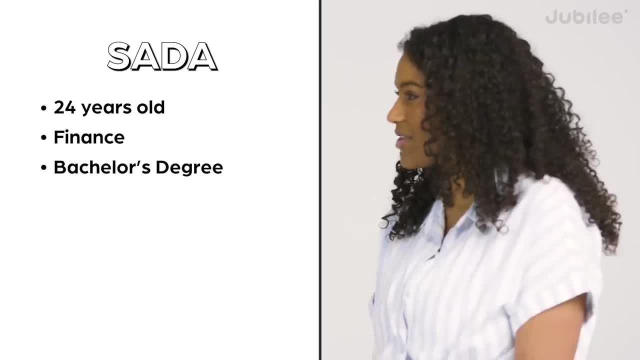 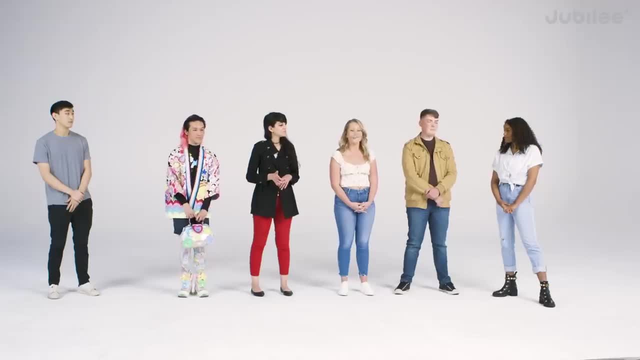 I'm Sade, I am 24.. I work in finance. I have a bachelor's degree. I went to Yale. I'm Tyler, I'm 21.. I'm a high school graduate and I work in the Marine Corps. I'm Kaylee, I'm 25.. I'm a software developer. I went to Ohio University and I have a bachelor's. 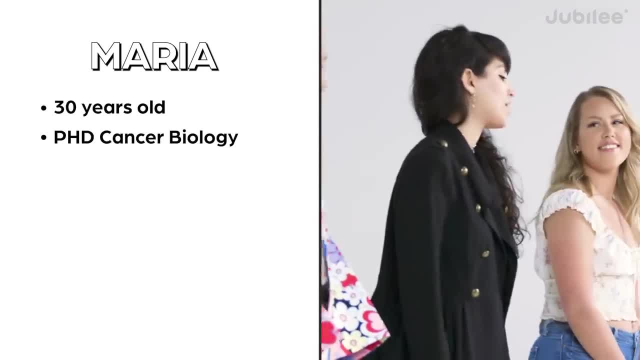 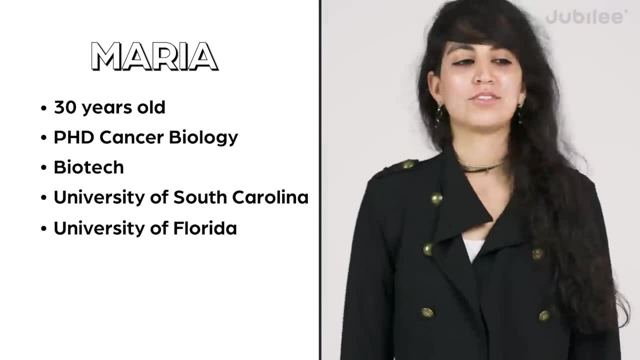 degree Maria. I'm 30 years old. I have my PhD in cancer biology and I work in a biotech industry. Grad school I went to University of South Carolina and undergrad I went to University of Florida. Hi everybody, My name is Sean, I'm 27.. 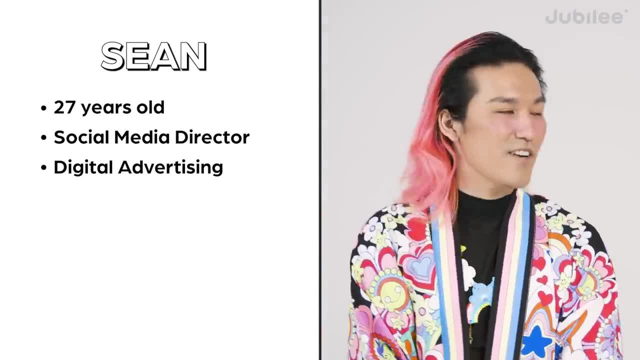 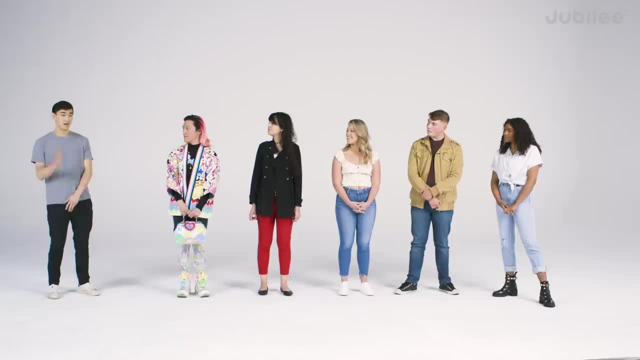 I'm the director of social media for our company and I also work for a ZUAT ad agency. I got a double major in dance and cultural anthropology. Undergrad I went to Loyola Marymount University. Hi everybody, I'm Ray, I'm 24.. I graduated with a bachelor's degree in Harvard recently. 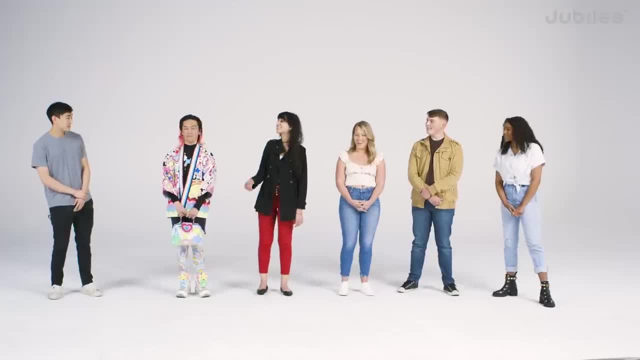 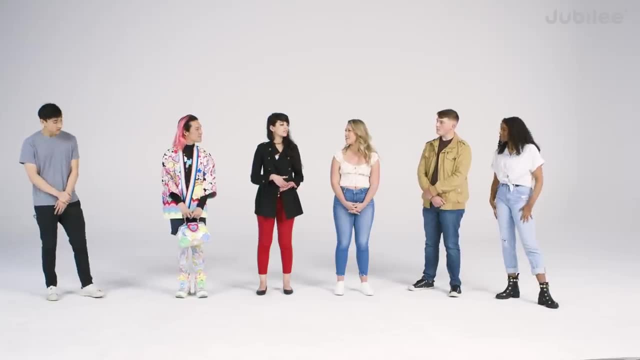 And I work in consulting. Oh, they're babies. I know That's what I was saying. Is age a factor? Yeah, it gives you like years of experience. Awesome, We need a. maybe it's good to identify what intelligence means to everybody. 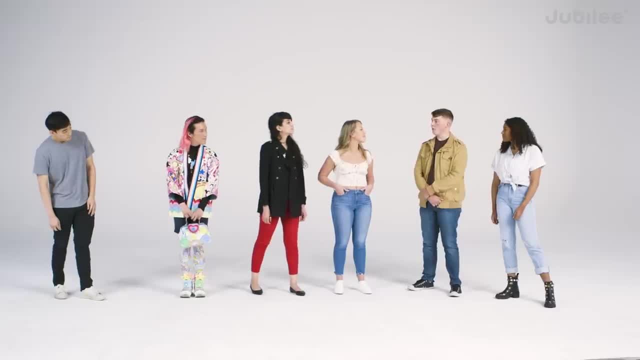 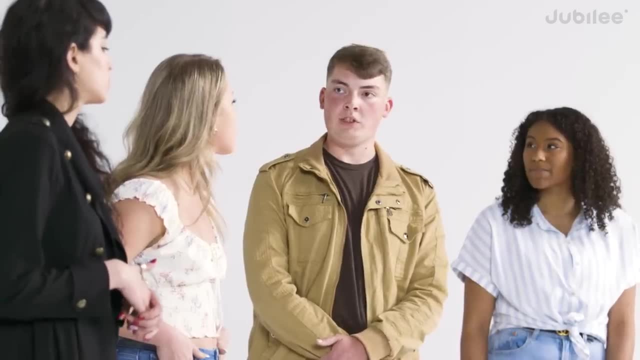 I think intelligence is better defined. It's your adaptability and your problem solving skills, more than it is your education, Obviously like the education, the stuff you've been through puts a lot into playing it, because it gives you more resources, more thoughts to draw from. 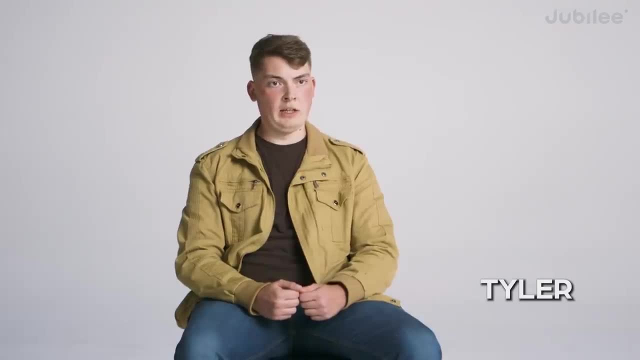 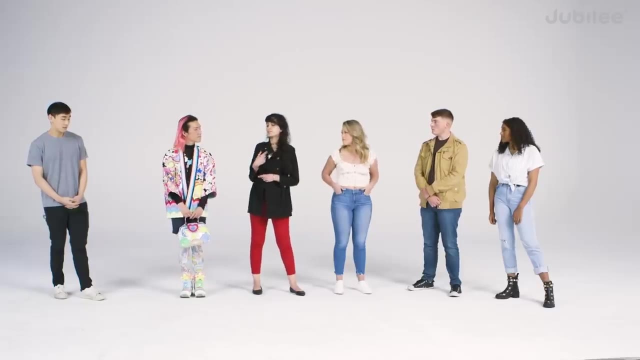 The formal education definitely helps, but I don't think it's in any way essential. So what is the most essential? I'd say, the most essential thing would probably be common sense. Yeah, so for me personally, I think intelligence is both EQ, IQ and that common sense street. 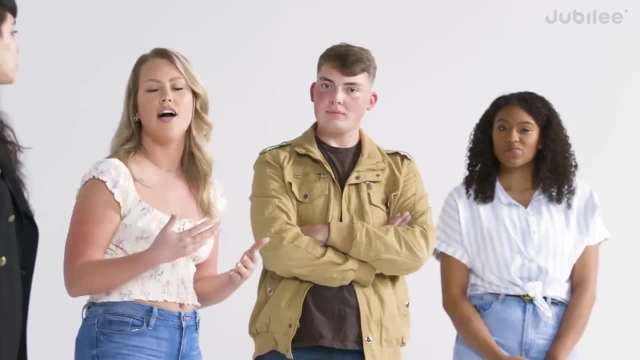 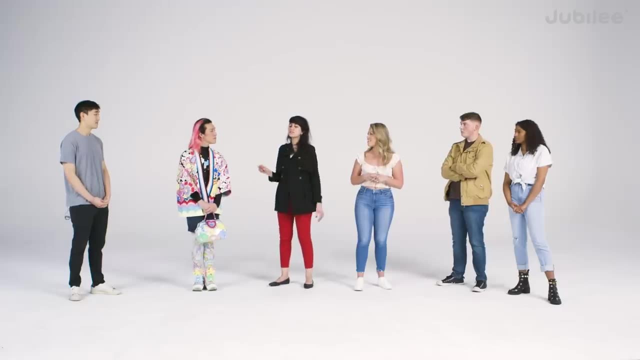 smart intelligence, all of that combined People, consciously or unconsciously, when they see someone form an opinion, they're going to take that opinion immediately, Like I'm sure we all did. right away When I saw you, I told myself, Maria, do not judge him just by his looks. 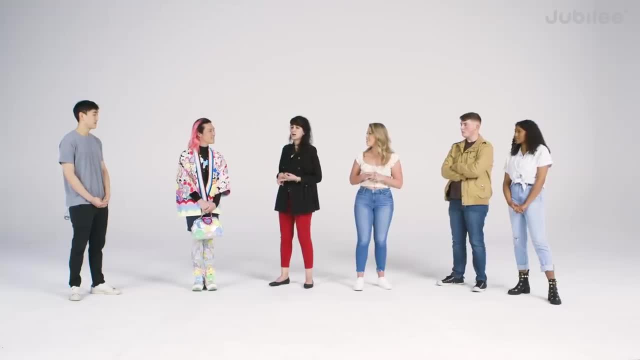 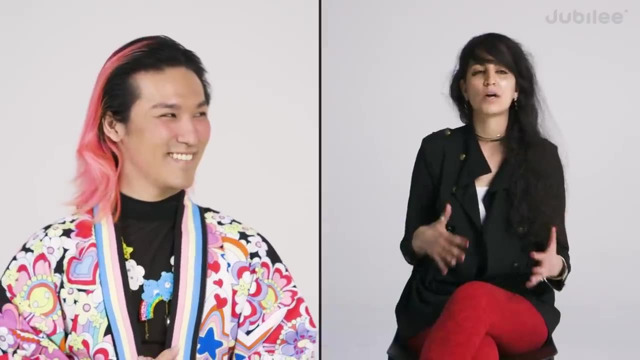 He could be throwing you off or that's just who he is, but he can talk to talk and walk the walk. Sean, I didn't want to judge him based on the way he looks or dresses or acts, So I was like I think he's intelligent. 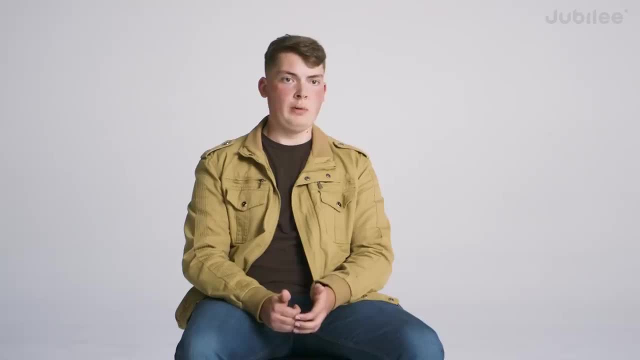 First impressions. I would put him at the bottom only because when I was in school, all the other people with like the bright neon colors and stuff, they were typically the ones doing worse in classes. If we were ranking confidence, I'd definitely put Sean. 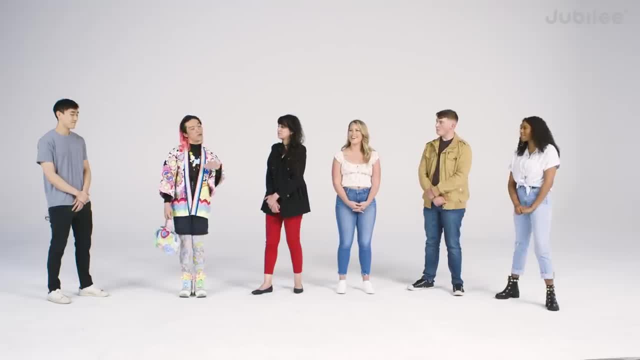 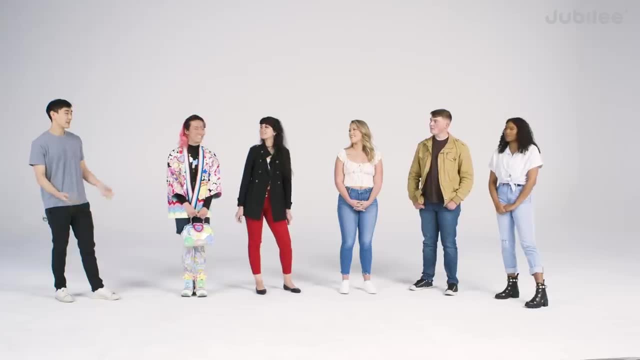 Yeah, I would put Sean on it very first place. So what is the definition that we're going with is the biggest question. I like your definition. I know I was going to say I like my definition. It combines everything. Does anyone have any like initial? 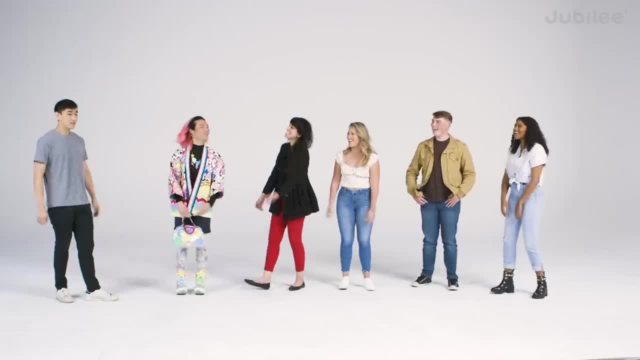 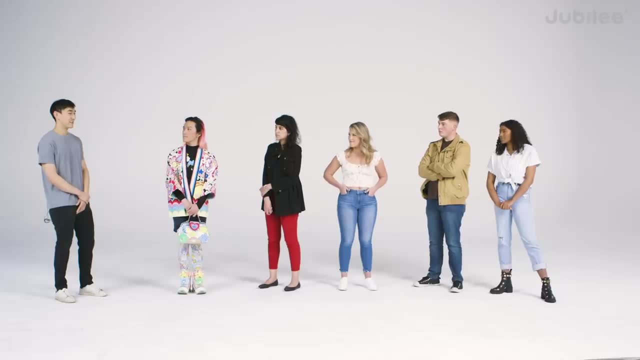 You can be honest Start on that side. I'm done going first. I feel like I have a good combination of both, like book smart and street smart. So, yeah, I think I have some input on that. There's so many aspects to intelligence. 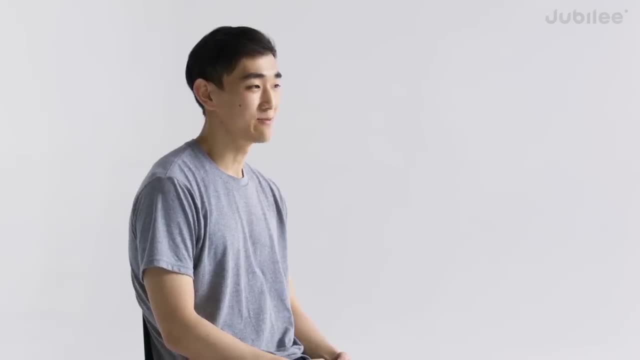 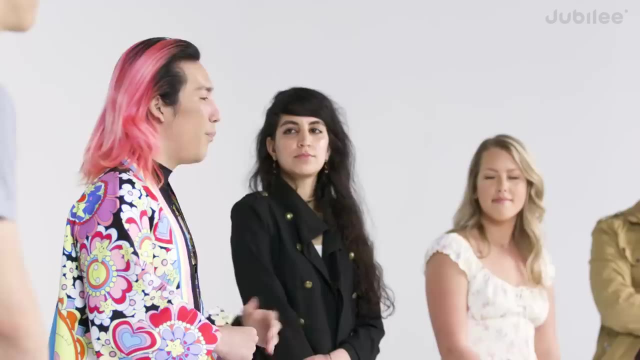 It really goes beyond IQ and EQ. Even those two different things, Different factors, really don't really capture what it really means to be intelligent. I know I'm not, you know, from Yale, I don't have a PhD, but what I lack in those areas? 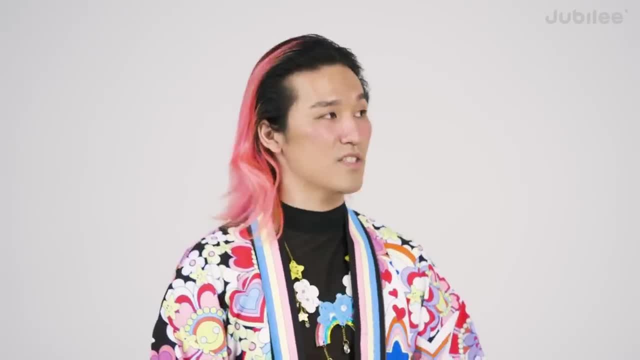 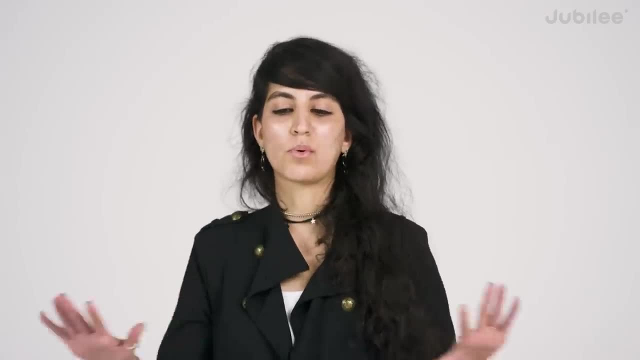 I'm able to still problem solve and use my own skill set, my emotional intelligence, as well as my social intelligence. Besides my education and background, I feel like I have high like emotional intelligence, Like I'm aware of my surroundings. As a software developer, my problem solving skills are obviously top notch. I think I 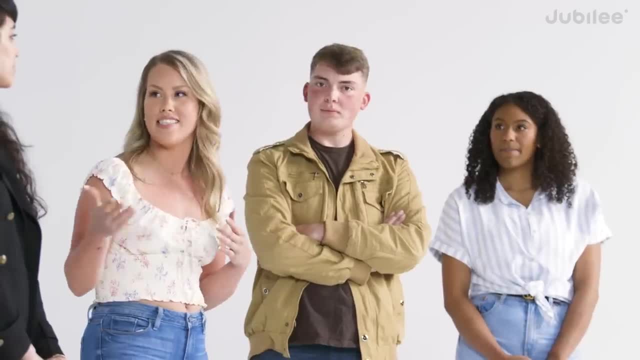 would say My whole life I've kind of had to fight to be seen as intelligent. I think I'm so used to having to do that as a woman to just like step up and be like. you know I deserve to be here. 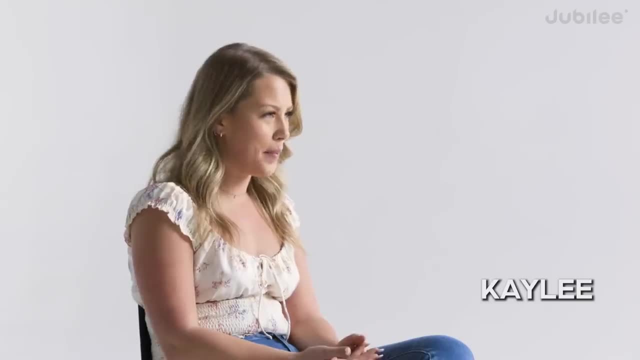 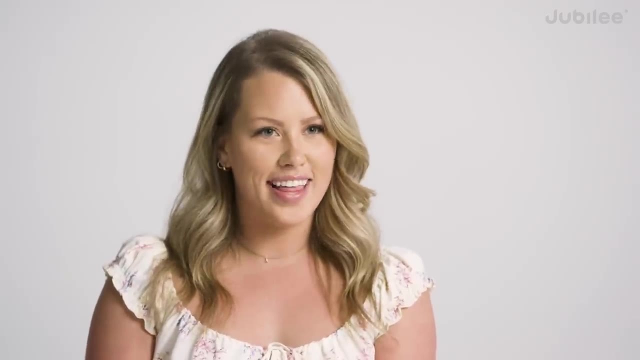 My first job out of college, I was working at a law firm. Gentleman came up to me and said: Hi, you don't look like somebody that would work at a law firm. You look like somebody I'd go on spring break with. 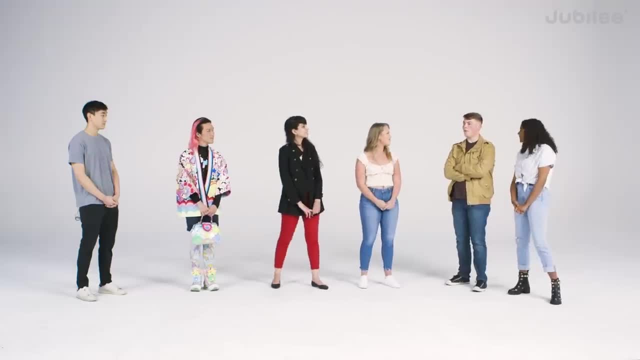 And I'm like what? Obviously, out of everyone here, I've got the least formal education. I consider myself intelligent, my mental dedication and my ability to adapt and to problem solve. What I do in the Marine Corps- I'm a seabird defense specialist. 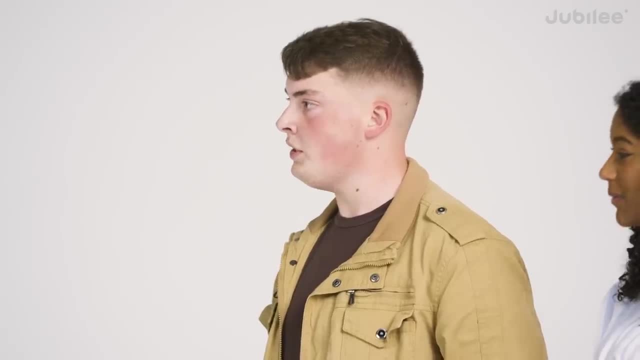 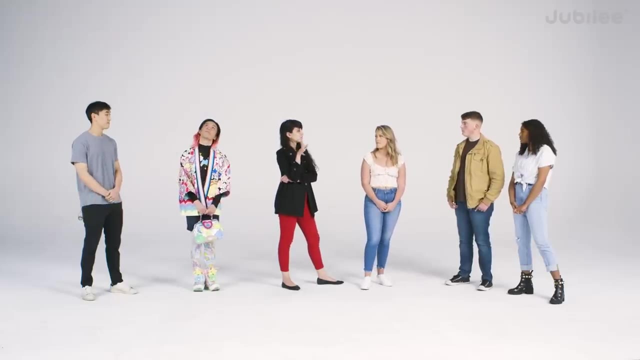 I think that, by virtue of what I do, that already requires some amount of intelligence. Sorry, quick question. So do you think that only certain people can do your job, or do you think anyone can do your job? Only certain people? You have to take the ASVAB before you go into the military. 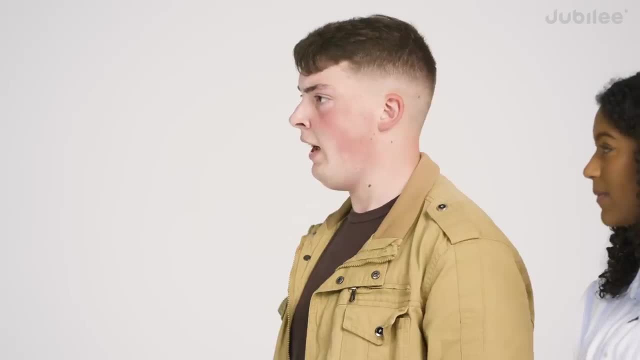 That's not really how much you know, but how well you can learn information, And I got a 94 on that. It's not an amount of how much you study. how much you know, You're not going to really get better at learning. 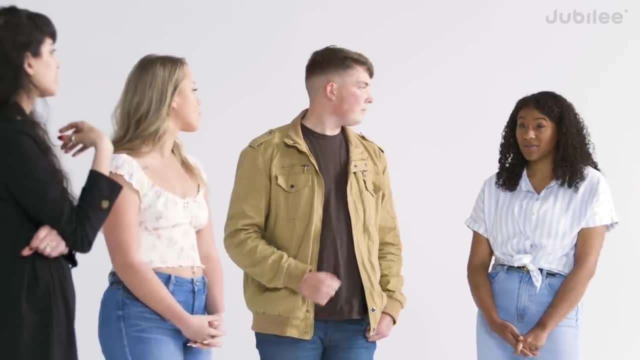 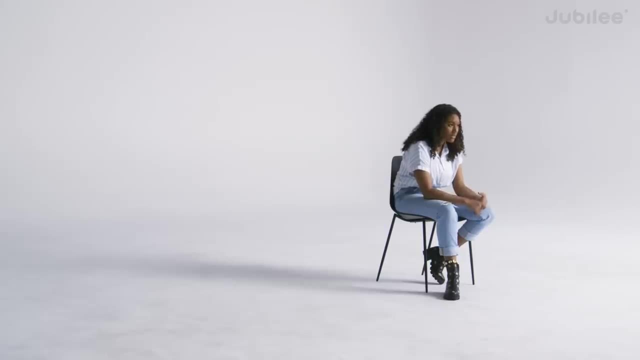 Does that make sense? I strongly disagree with You. don't get better at learning. The idea that you can get better at learning is a pretty big signifier of intelligence. I'm very much dyslexic, I have ADHD and I'm on the autism spectrum. 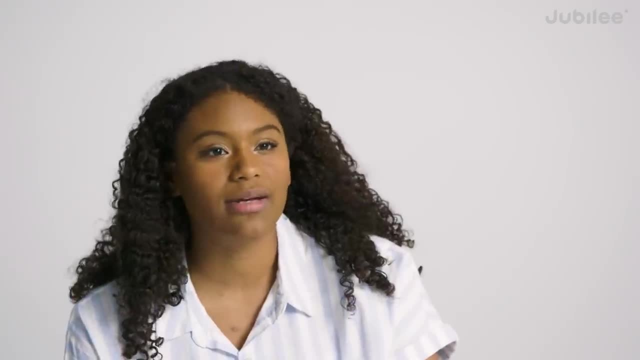 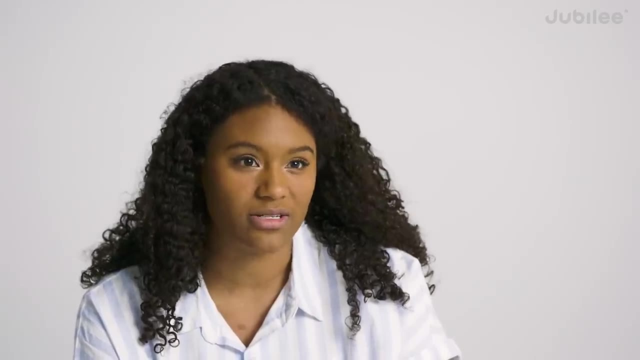 Dyslexia means that there's a big gap in comprehension, So I was scoring 99th percentile in certain areas and like third percentile in others. I'll never be able to learn another language. I took Spanish for 12 years and I can still basically only order a burrito. 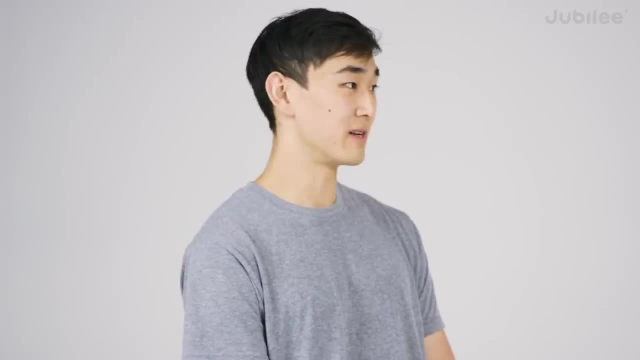 So I have a question: Why did you go to Yale and why did you go to Harvard? My parents are immigrants from China. I'm a first generation immigrant. I'm a first generation immigrant. I'm a first generation immigrant as well and college student as well. 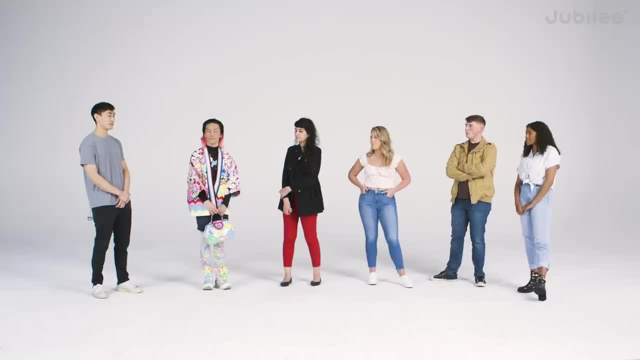 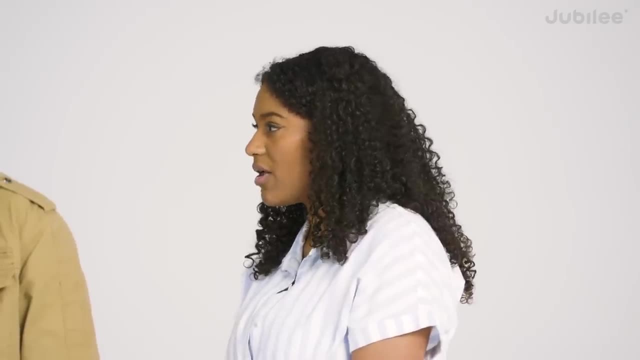 My family always really stressed the importance of formal education. For me. that was something that I really strived for. I wasn't planning to go to college. I didn't. That wasn't like a goal of mine. My parents were like, well, you should apply to at least one college. and I was like I'll 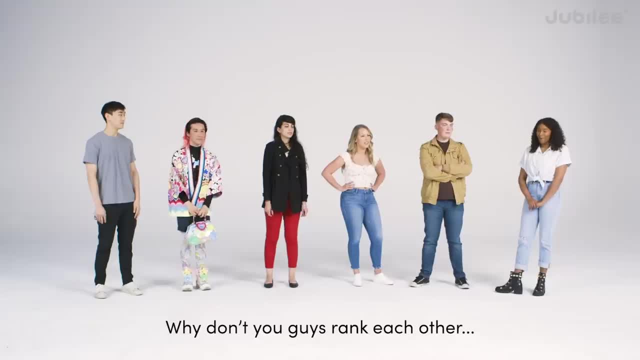 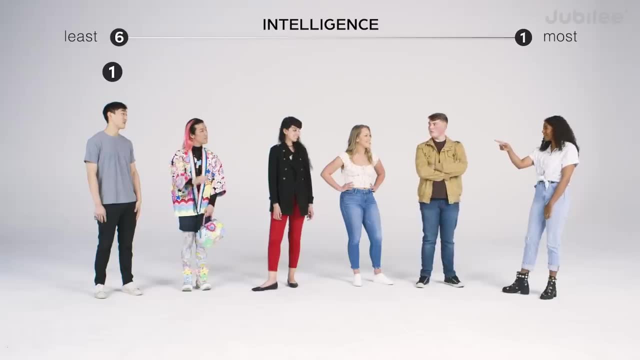 never get in here. And then I went to Yale. Why don't you guys rank each other from one to six, including yourself, and give reasons why you want to do what you're doing? I got to go one. No, Oh yeah. 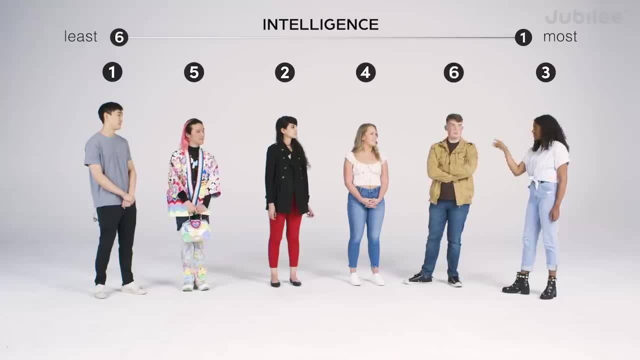 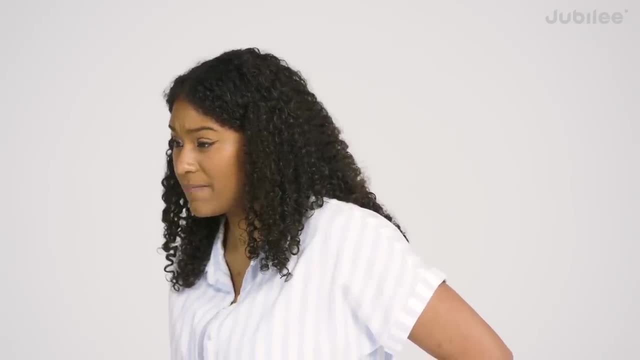 Two, Three, Four, Five, Six. I would rank you as a six, Not meaning that you're not intelligent. I also think that I don't place a lot of value on the military Period. No, that Yeah, Full stop. 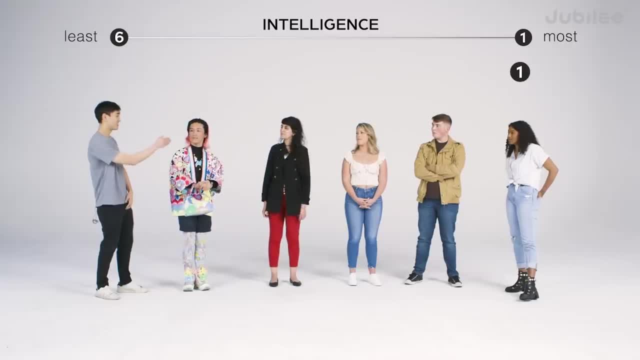 I'd probably do one, two, three, four, five, six. I'm sorry, I'm the villain this episode. Does anyone think they're like either end of the spectrum? I'd say I'm one, if nothing else because I know what I'm doing. 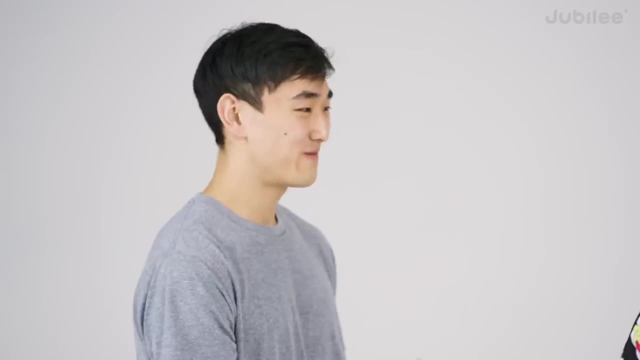 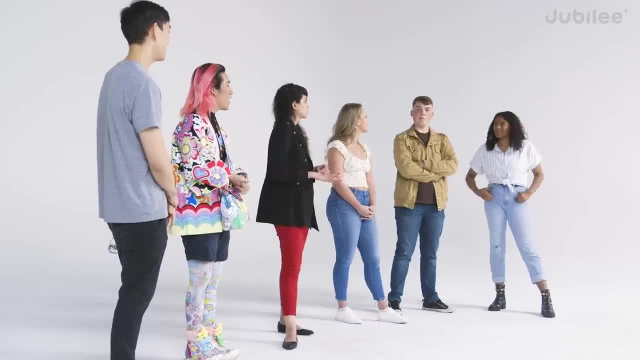 I know what I'm doing. I know what I'm doing. I'm the villain of the spectrum. I'd say I'm one, if nothing else, because I know what I'm about and I'm sure of that. Wait, You guys have to rank everyone too. 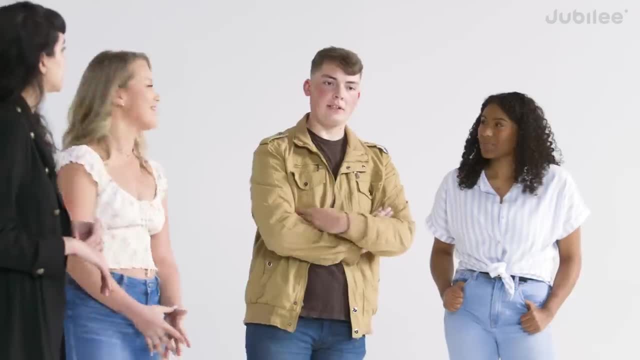 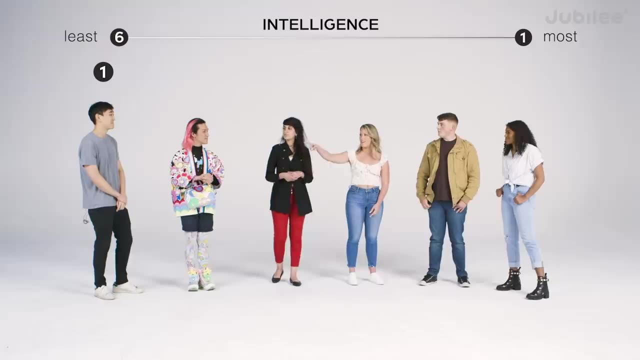 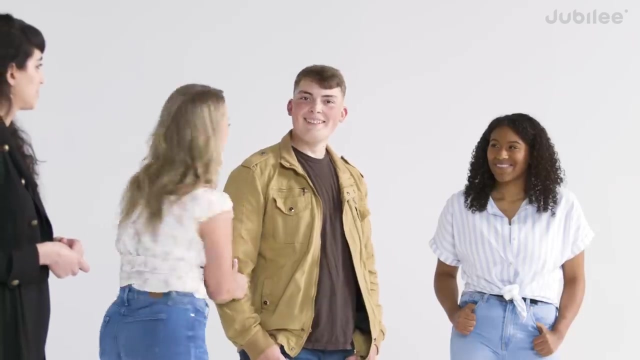 That is so unfair. No, no, no, no, no. I would say one, two, three, four, five six. Okay, I think, one, two, three, four, five six. I'm sorry, I'm sorry. 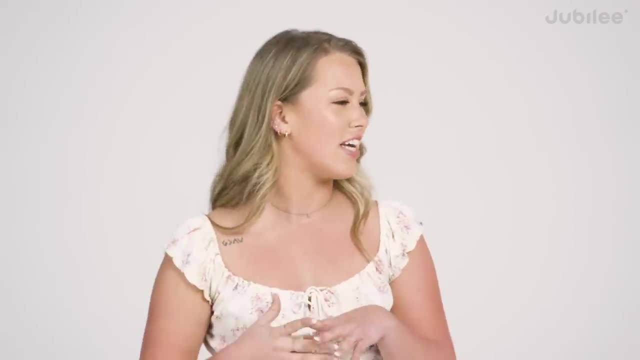 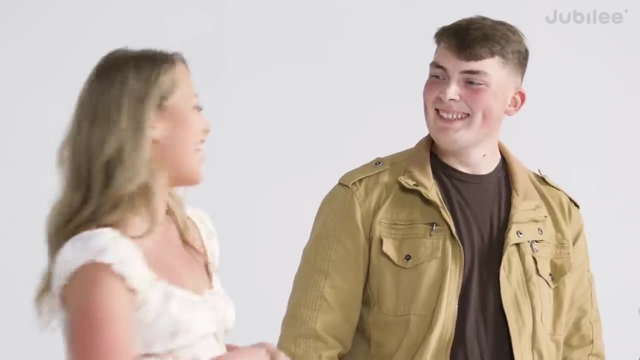 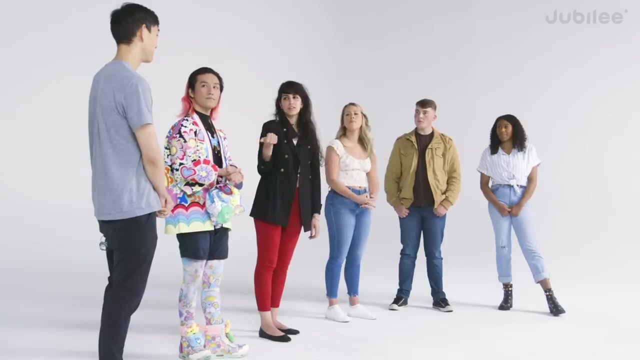 It gets hard for me to look past the education Part going to college. I think you learn a lot, if nothing else emotionally, but I still think you're smart. one, two, three, four, five, six, One immigrant parents, first-generation going to college: humble, modest to me. 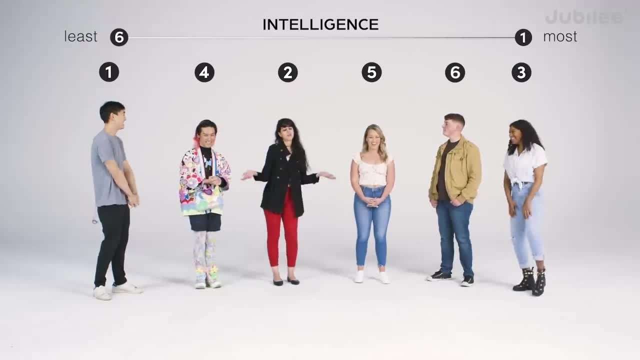 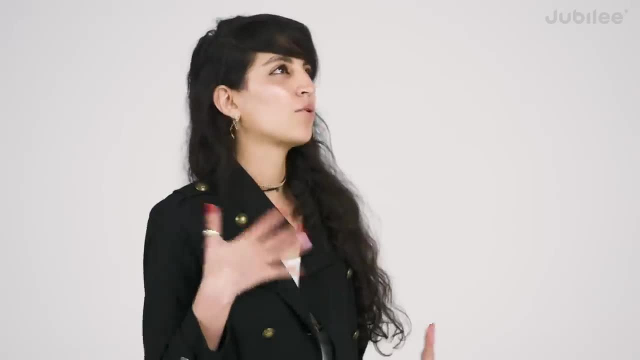 I don't know PhD cancer biology scientist. I work in a biotech company. We make COVID-19 testing kits, stuff like that, And then six. it has nothing to do with your background. I don't think you really have the highest EQ out of all of us, Tyler. 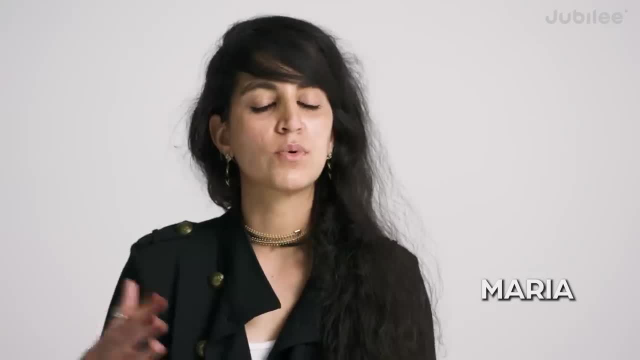 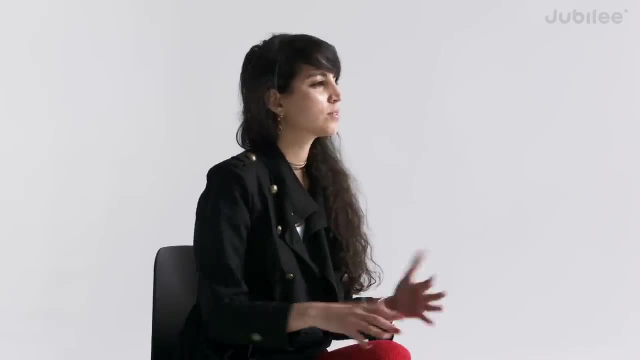 He ranked last, for me personally because the way he carries himself. He was ranking intelligence based on his point of view and not taking in other people's point of views and compiling results, But really just came down to his body language, his demeanor, the way he carried himself, the way he acted towards the group. 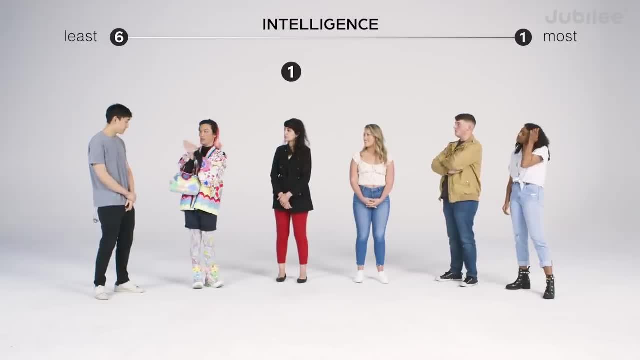 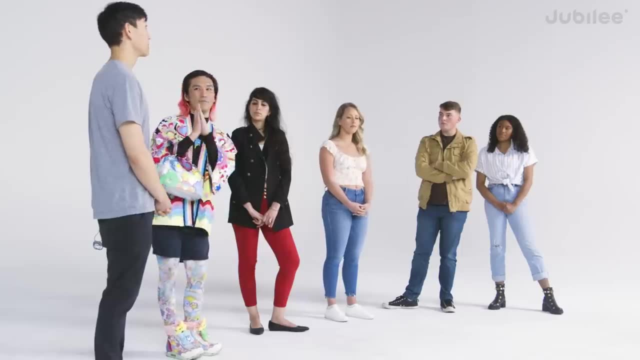 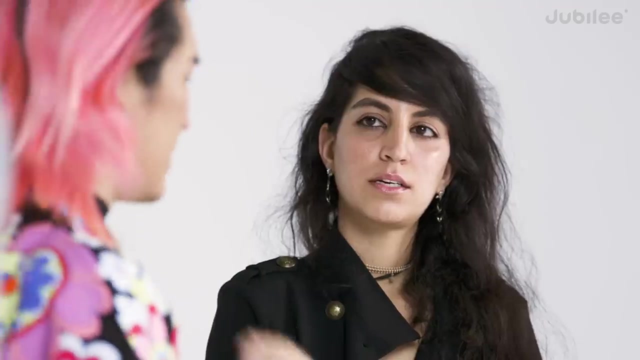 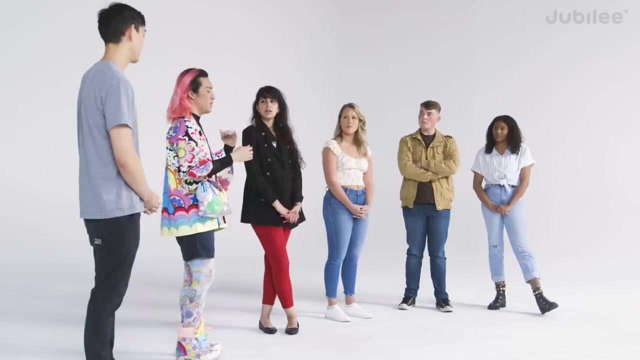 I would put one, two, Three, Four, five, six. So The reason why I put you a number one is I think you have the highest not only EQ score out of everybody, but the way you present yourself as well as being a PhD student. I think it's just like a huge thing when I put myself six, because I feel like I might be the 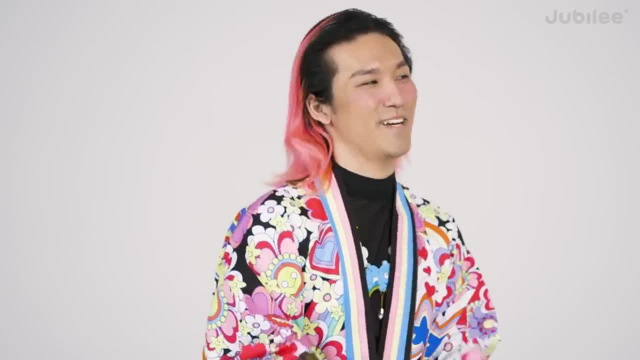 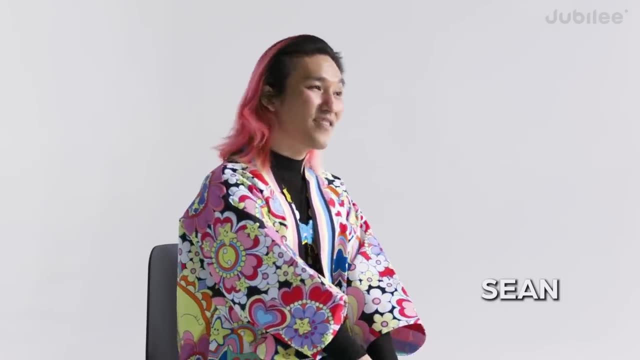 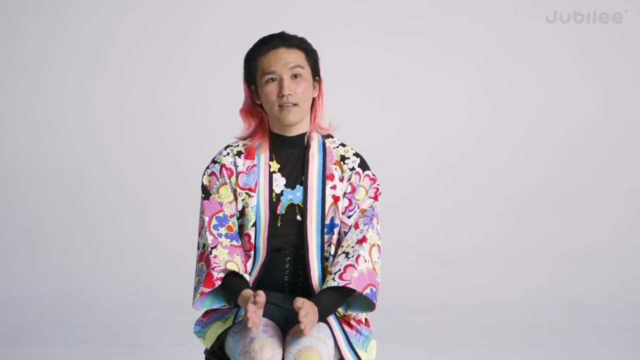 Weakest in terms of actual IQ score. Hopefully I can make it up everything else, So I did put myself as least intelligent. However, if it can't be me, I definitely think Tyler. unfortunately, his way of thinking is Linear and I think intelligence is almost like a sphere. 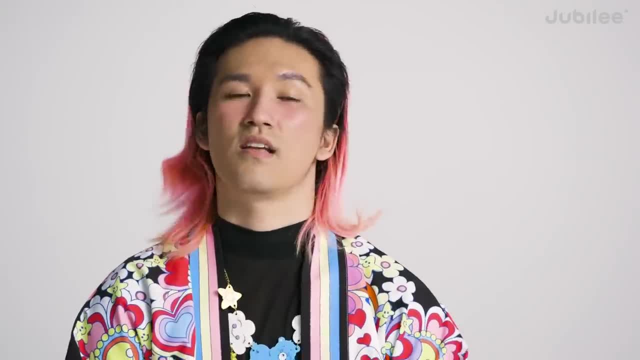 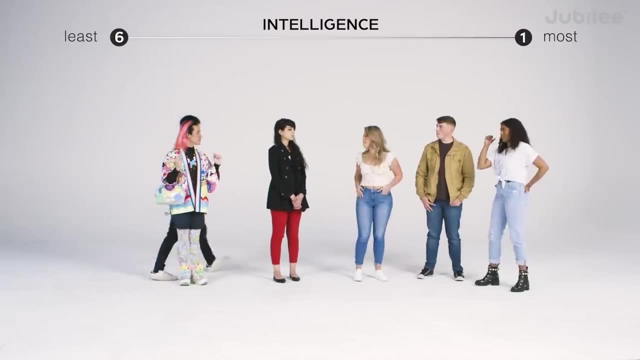 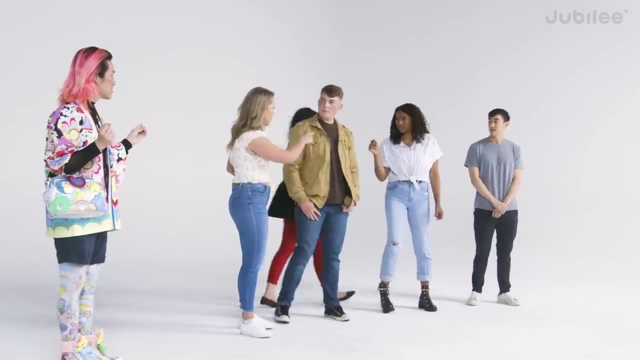 It's a picture and right now he's only coloring with one color than you know, with the rainbow. So who got the most number ones? Thank you, Who's down? who got the most? I feel like you were definitely three, right? Yeah, I mean between you and Tyler. 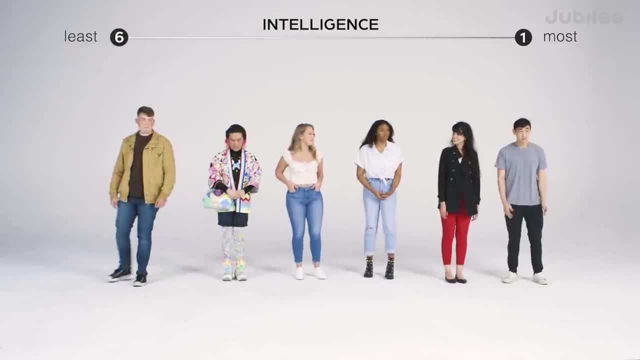 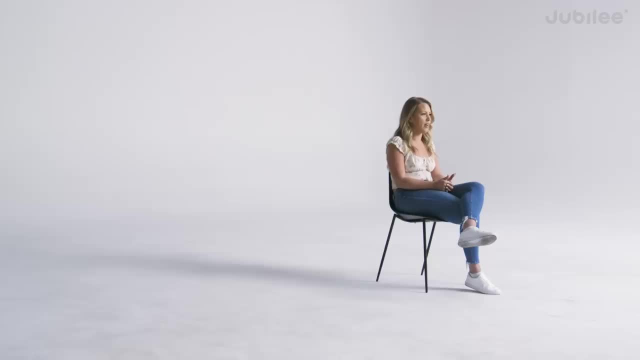 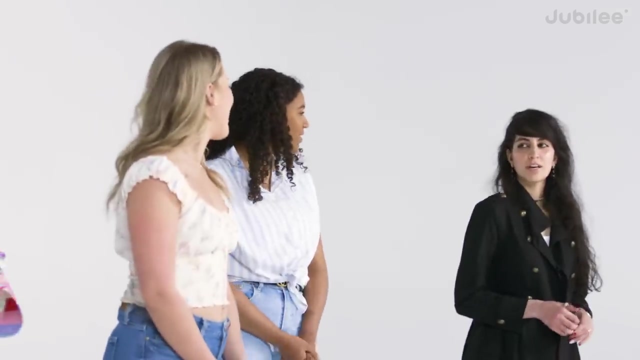 You were four and I was five. Sure, I think that I sort of expected to be ranked a little bit lower. at first glance and first interaction with me, It's hard to tell how intelligent I am. It's hard to tell how intelligent anybody is. is anyone upset with where they're standing? 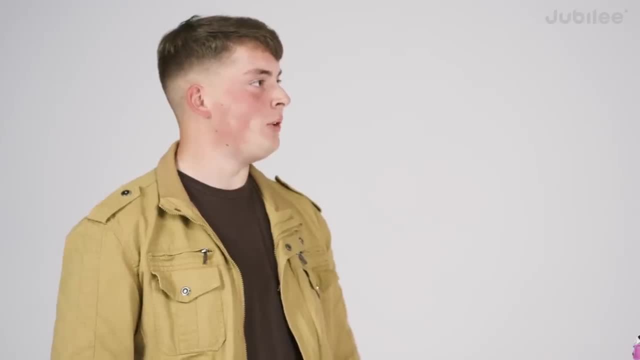 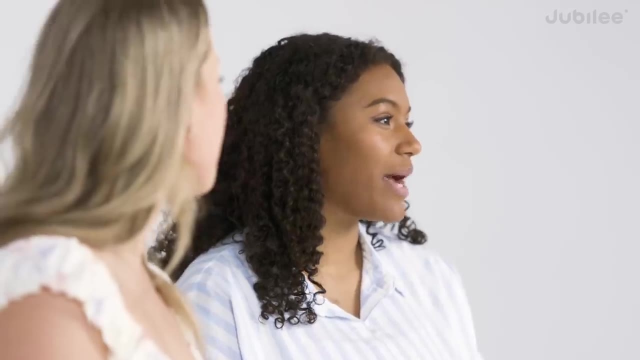 I think it makes sense that I'm down here. like the guy graduated from high school and then joined the military. He probably wouldn't be like high up on there. if I was in their shoes, I definitely would have also ranked myself among the lowest. I do feel like there might be a prejudice acting in terms of ranking you. 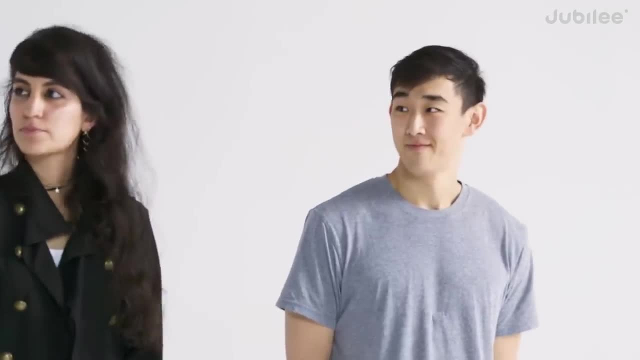 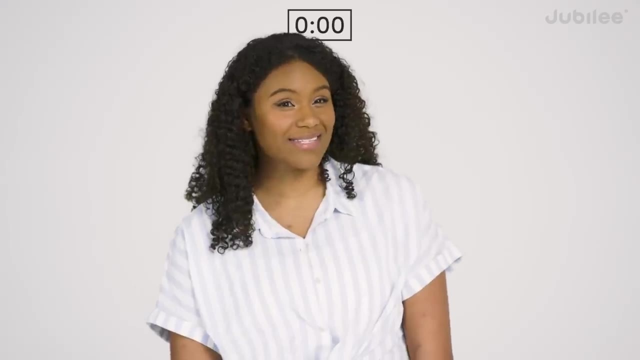 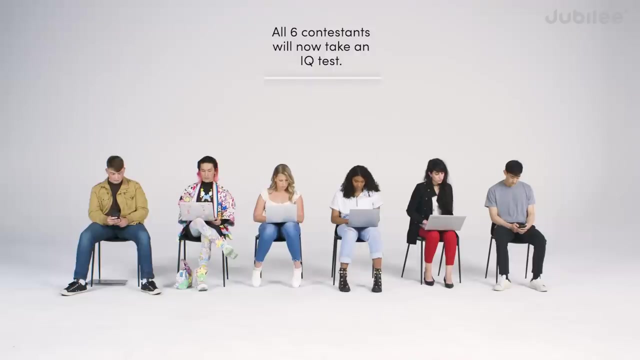 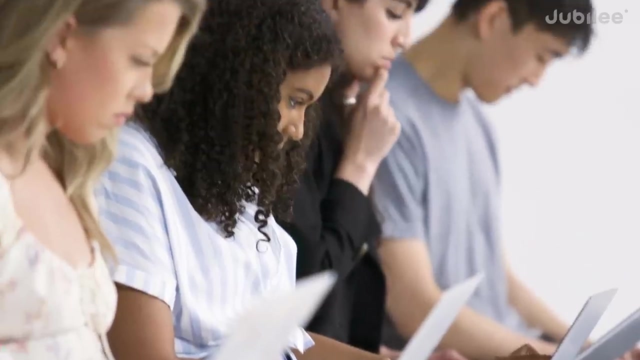 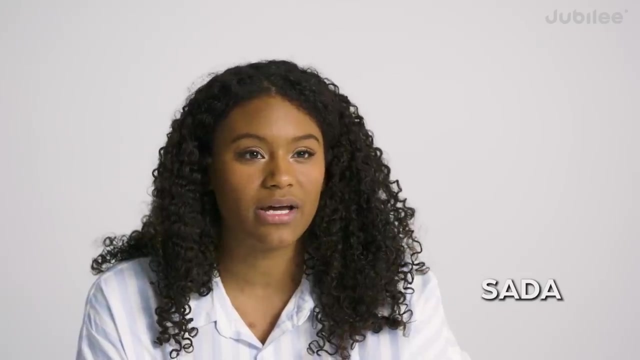 Okay, I was thinking that too, But I agree with the ranking. I think you probably are the most intelligent out of all of us. I would feel weird placing you there and not acknowledging the dynamics in which we did so. Hearing that to take an IQ test was definitely hard to hear. quantifying things for me in that realm is really hard, because it gives you. 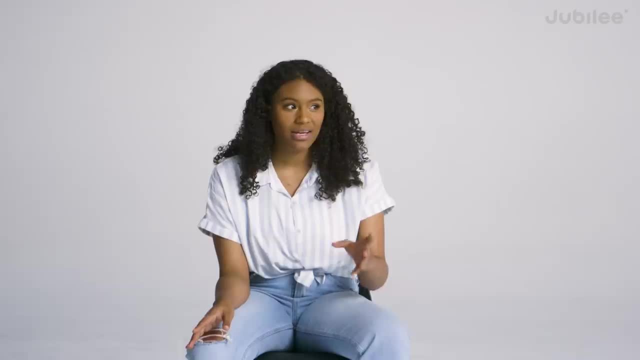 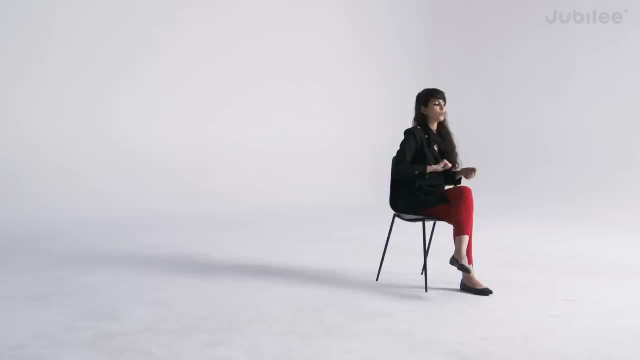 Something really solid. even if you don't buy into IQ tests, It still gives you a number at the end of the day, which is something you have to grapple with. I Literally thought, when you said, to open the computer, we're gonna look at social media, that I didn't think an IQ test would be part of it.